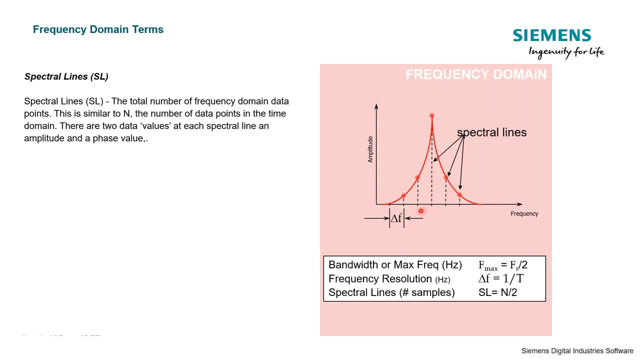 when we talk about the total number of frequency points here on our spectrum graph, it's similar to block size. Block size number of points in the time domain We're talking about now in the frequency domain, though, So these spectral lines will represent that, And at each. 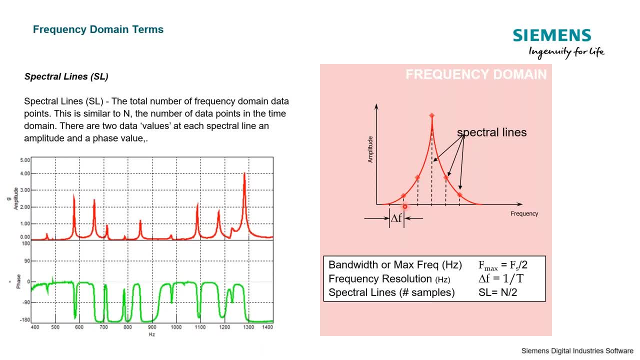 point. we actually have two values And that's because the fast Fourier transform. we get a complex number out of that. So it has amplitude and phase, or we can represent it as a real part and imaginary part And the spectrum line is going to be the block size divided by the time. 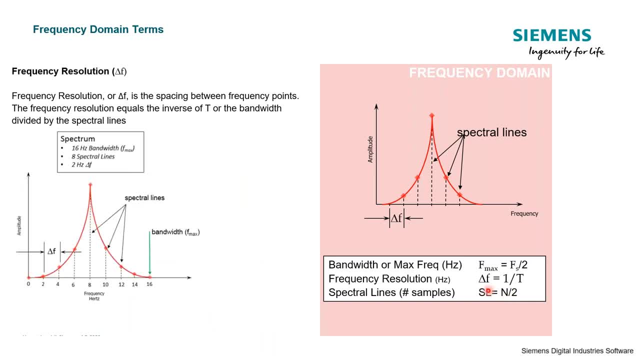 by two. Now, frequency resolution represented here is delta. f stands for our frequency resolution. It's one over our frame size And we can just think about it like this: If we had a bandwidth of 16 hertz and we had eight spectral lines, then we're going to have a frequency. 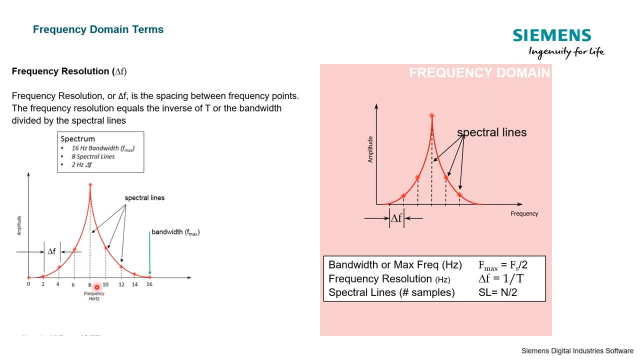 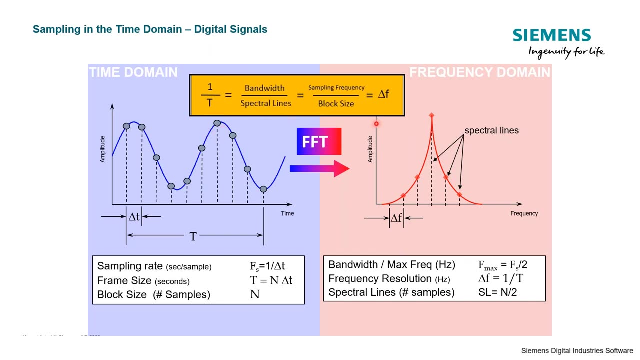 resolution of two hertz. right, The distance between each one of these spectral lines would be two hertz. So as well, we could rewrite that equation and just say that delta f is the bandwidth divided by the number of spectral lines as well, And I really like this slide in particular. 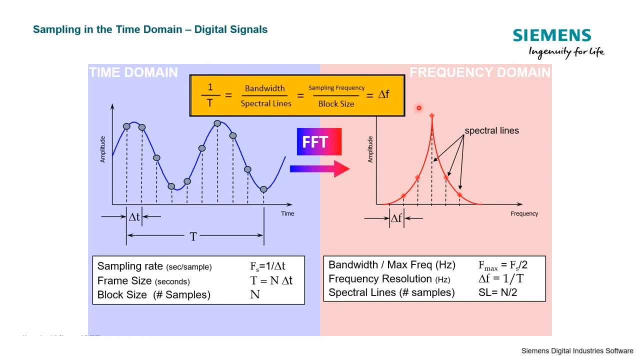 because it kind of hopefully relates to you or conveys to you the relationship between all of these parameters. we've been talking about the bandwidth and the spectral lines, the sampling frequency and the block size And one key point, this frame size, remember, that's the amount of 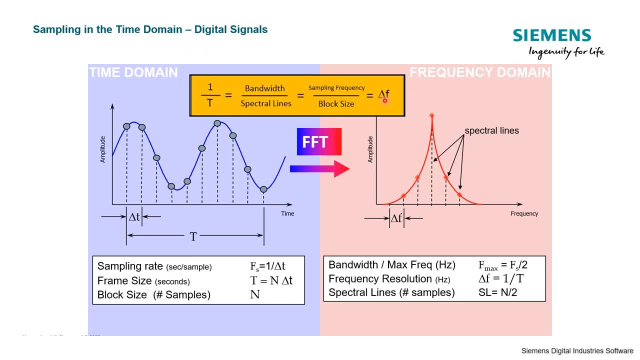 time we need for one FFT. If we want to have a really fine delta f, really small frequency resolution, then we need a lot of time right. Just for the one average we would need a lot of time. This needs to get large for this to get small right. So that becomes an important point. 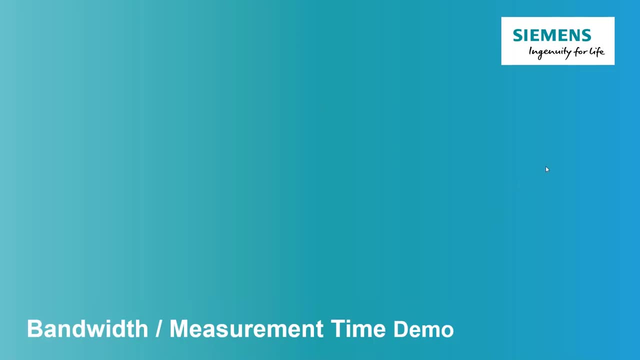 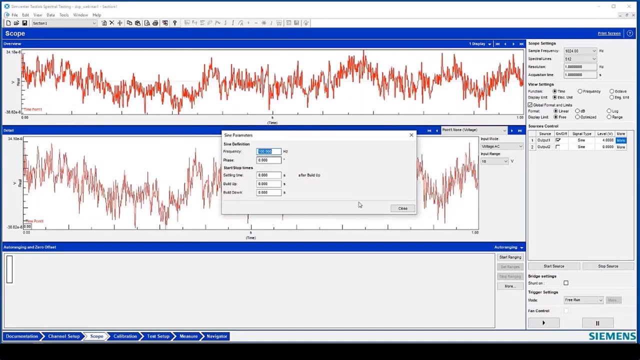 Let's look at another demo, though, to highlight this idea of bandwidth and measurement time. Great, And I thought I was maybe scaring you before, So I went in here and I changed the frequency of the sine wave I'm generating back down to 100 hertz or back to a nice-looking 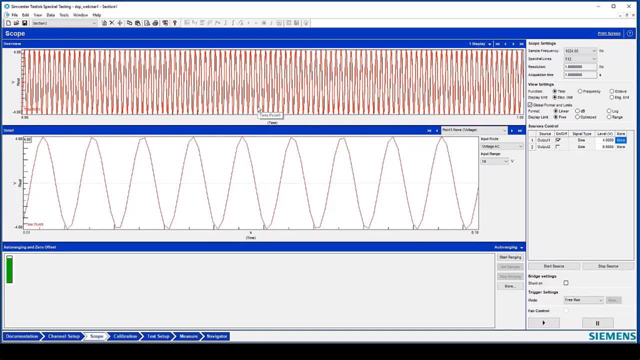 sine wave. So that's the frequency of the sine wave I'm generating back down to 100 hertz. Good for you, Charles. Yeah, I'm happy. Okay, And you can see up here. I got those settings you were talking about, I got sample frequency, I got spectral lines And in fact, I think, on your 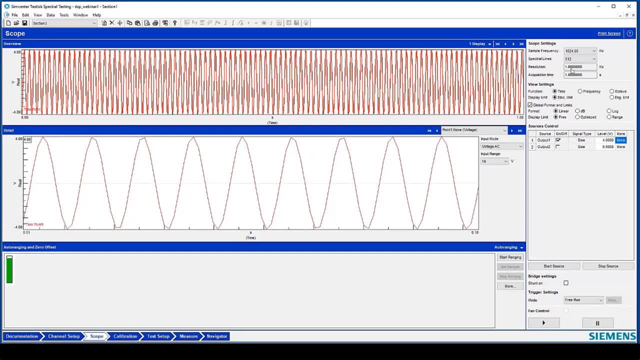 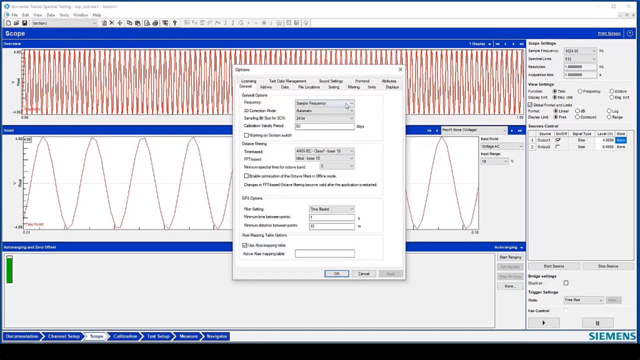 equation. it actually said: bandwidth divided by spectral lines is your frequency resolution, And then there is your acquisition time. I'm going to go here back to tools options. I'm going to switch this back to bandwidth or max frequency, So instead of 1024, what this is. 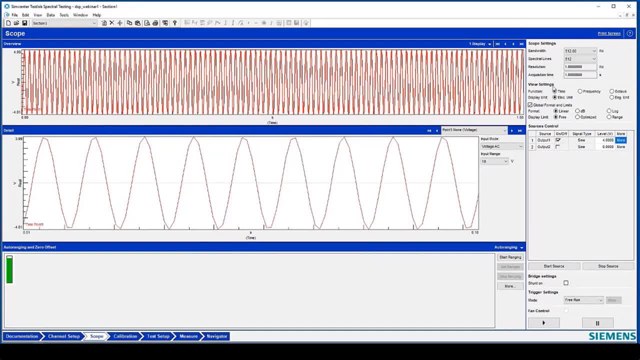 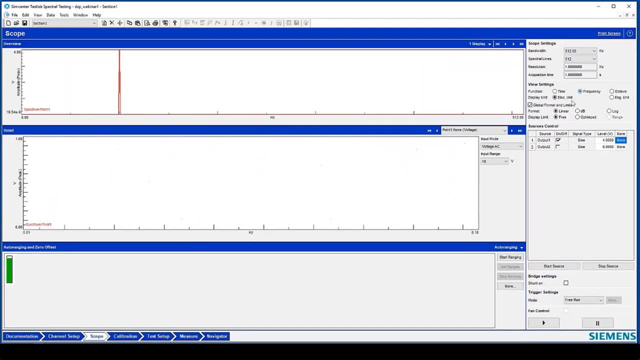 saying is: I can see 512.. That's my max frequency. I'm using 512 data points to digitize it, So like if I look at my frequency spectrum here, So I can say marker style, cross here, so that we can actually see. 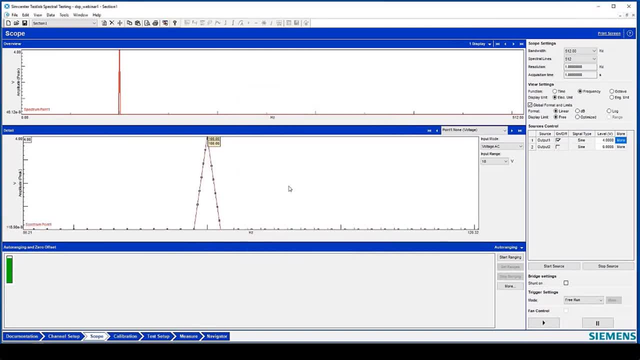 those data points again. I'm going to zoom in. So I got 100 hertz, 4 volts. But what's kind of weird is, if you look at this, you can see that the next data point over. well, this doesn't go. 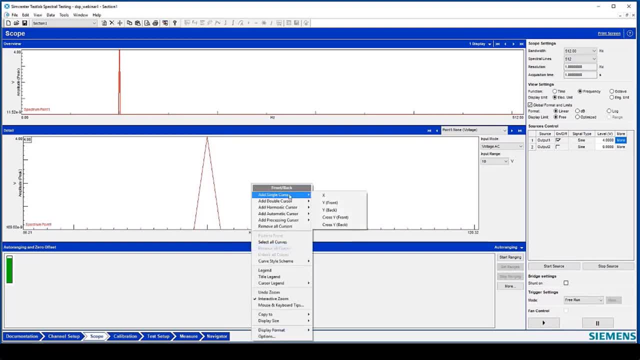 right down Here. If I put a cursor on and I right click on the cursor, say snap to data values so it doesn't float in between. you can see, at 100, I'm at 4 volts, Over here, at 101, I am at zero or something. 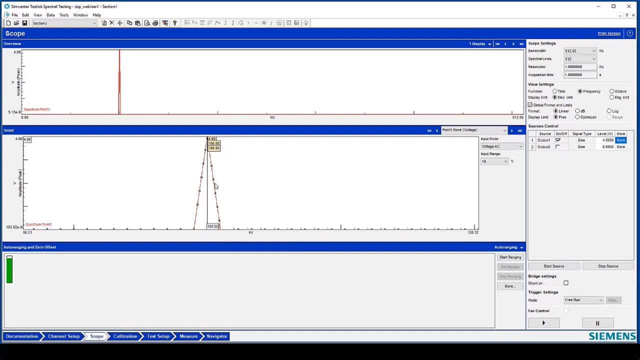 very close to zero And then it's zero from there out. There's really no data in between, It's just connecting the line. So what I have is: you can see I've got a lot of data, I've got a lot of data. 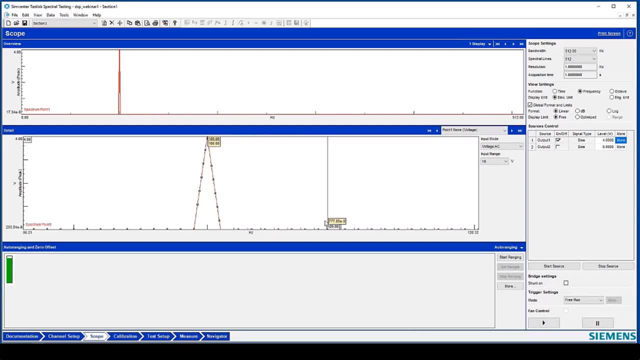 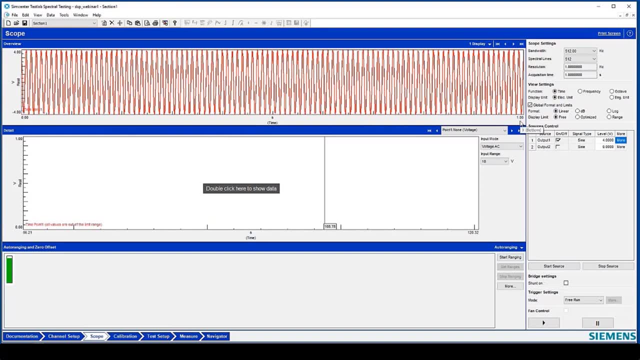 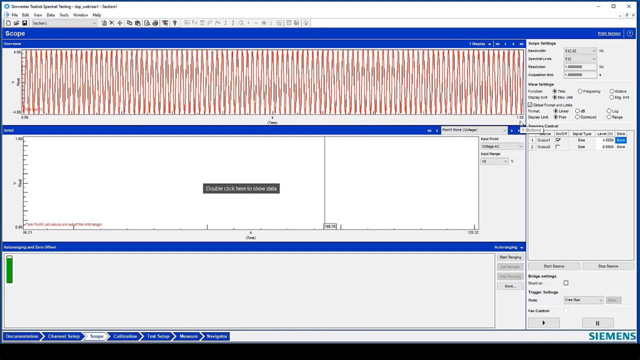 here it goes up to one second. Now maybe I'd be like: oh, I'd like to see that little finer frequency resolution. So I would go up here to 512 and increase the number of spectral lines. So if I double that now I got half a hertz of resolution. 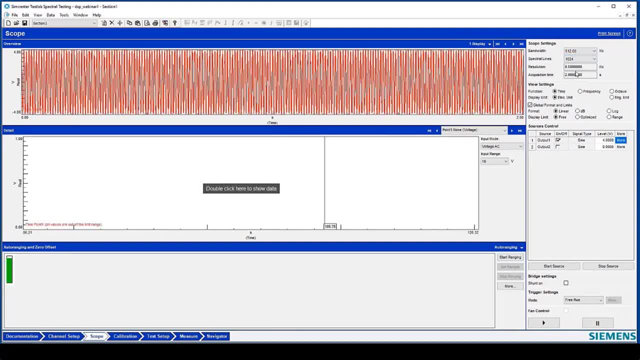 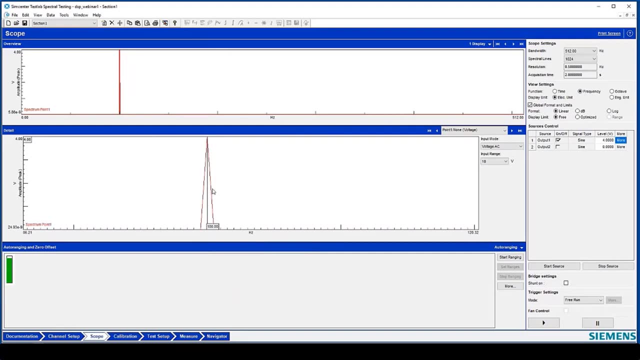 just these numbers divided and now the time domain is two seconds, so I have to take a longer chunk of data in order to see that's at a half Hertz. so now, as I move my cursor around, notice it's going a half a Hertz at a time. can you see that, Charles? yeah, yeah, pretty nice, huh, yeah. 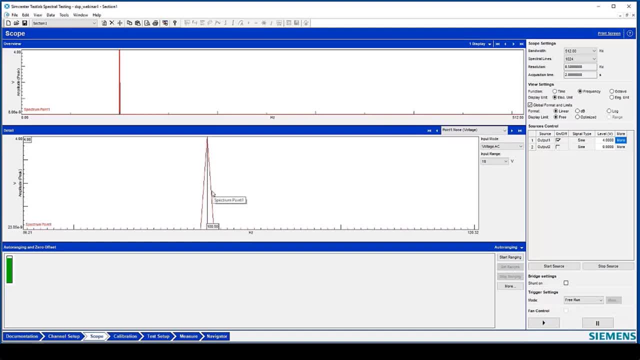 yeah, I like the point too that you're pointing out that, uh, the lines, the way it draws. when you snuck into the data points, there's all your for all your energy, that the 100 Hertz, yeah. so then I might say, gee, I want the finest frequency. 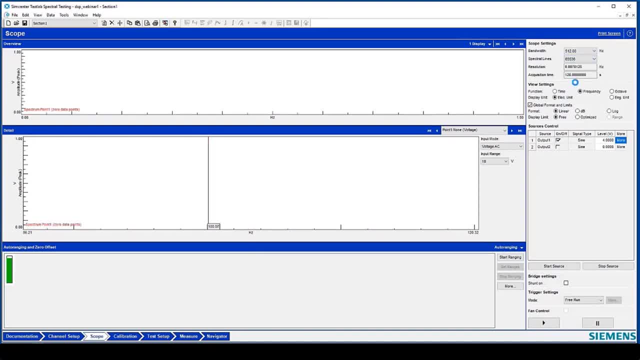 resolution possible. I could do something like this: guess what happens? how long is my acquisition, Charles? a really long time, yeah. two minutes. yeah, I think when I, when I first joined the company, I was working tech support one day and guys like you know, my system seems to. 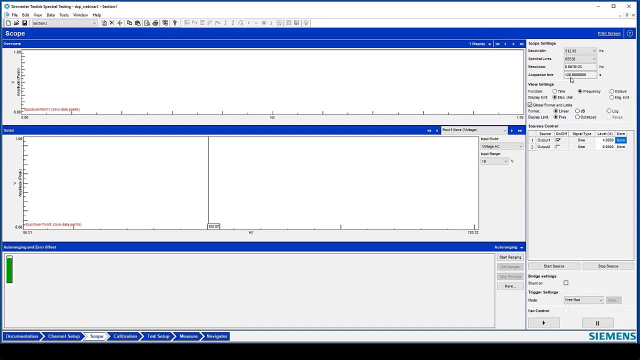 have locked up. I used to show the FFTs really quickly, but now it's like they can forever. it doesn't even come back. nobody had done Charles. he had a really really fine resolution. yeah, just crank it up the resolution, thinking hey, this thing will still respond at the same rate. but yeah, these things, you know it's. 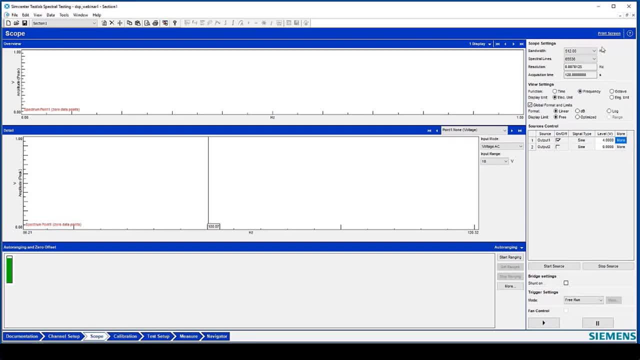 in some analyzers, other systems, and it's true of all digital signal processing or data acquisition systems- that inverse relationship. you may not even see or know that the acquisition time had to be increased greatly in order to accommodate spectral resolution that you required, so you could get potentially strange behavior. maybe I'll go for. 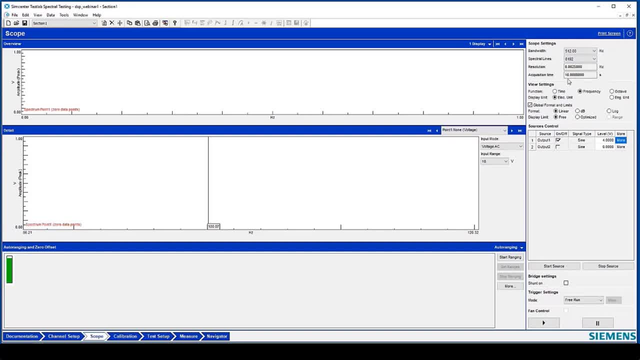 something that's a little less than 128 seconds. so now, after 16 seconds, I should see the screen update. so it's, and that's the time it takes in order to grab one chunk of time data to get a frequency resolution of 0.0625 Hertz. so you can see, there it came back. so yeah, that. 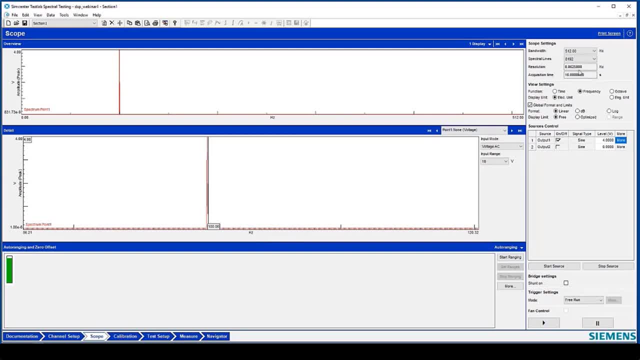 that relationship dictates a lot. if you want this 0.06. if you have, you have a Ferrari, right, Charles? isn't it to like 0 to 60 in 4 seconds or something? my hot wheels is variable, it depends on how fast I push it down. okay, so 16 seconds. 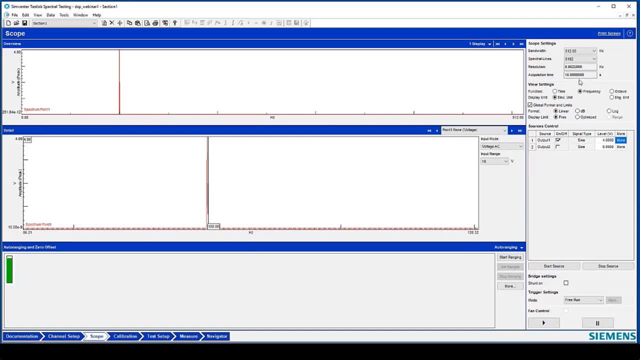 for Ferrari. that FFT is gonna be kind of a you can't even you get a run-up. you could get four run-ups in or something. yeah, maybe five, yeah, so, like you said, I think you said something like- yeah, you got to be aware of these settings and